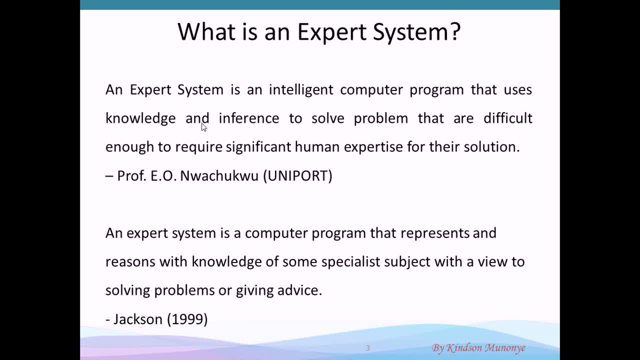 Now Professor EO Majukwu and the University of Port Harcourt here in Nigeria gave this definition. I heard a student ask a question, say: are robots expert systems, Or the assembly line for automobiles are they expert systems? Well, the professor asked the student: what is an expert system? 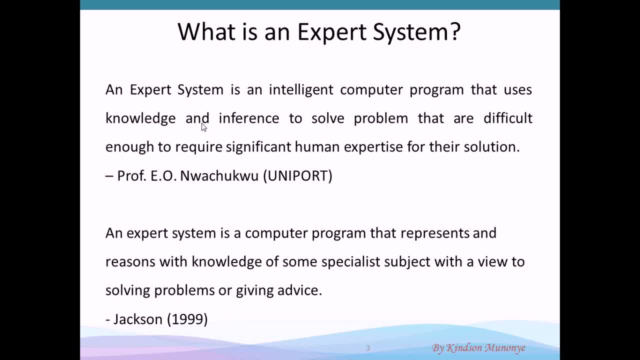 The student replied: it is a computer program. So expert system is not the hardware, but the computer program that makes it work. Okay, So the next ingredient in the definition says it uses knowledge and inference. Now, in an expert system there must be two ingredients, two components: the knowledge, that is the knowledge base, and then the inference engine. 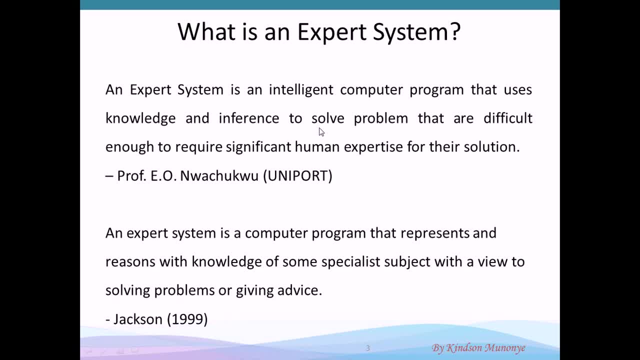 Okay, take note of the next part of the definition. it solves problems, but not just any kind of problem, Problems that are difficult enough to require significant human expertise. So it's not just simple problems. and then you say: I use an expert system. 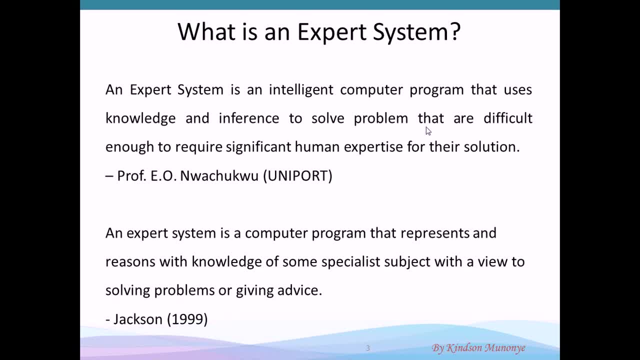 The problem will be difficult enough to require human expertise. So an expert system is a clone- okay- of a human expertise, a computer version of the human expertise. Now take note of another definition: An expert system is a computer program. 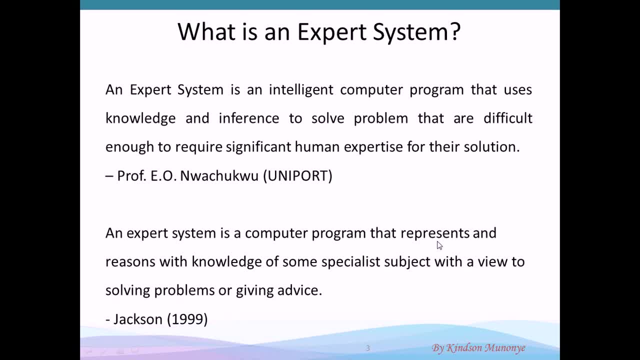 It tallies to the definition given by the professor here that represents and reasons with knowledge of some specialist subject with a view to solving problems or giving advice. All the same, the main point is it's a computer program. it solves problems, it uses knowledge. 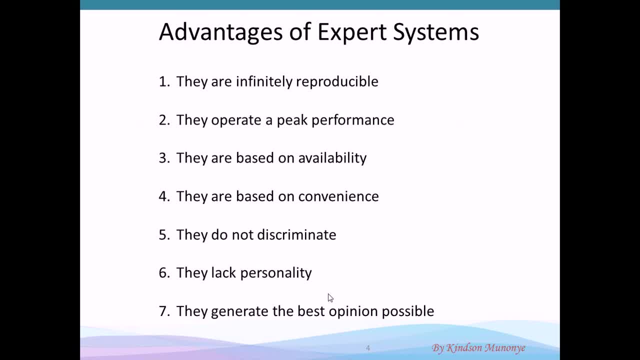 Okay, let's proceed. What are the advantages? Maybe you pause the video and take note of the seven advantages I have highlighted, But I want you to pay close attention to this one. It says yeah, number one: they are infinitely reproducible. 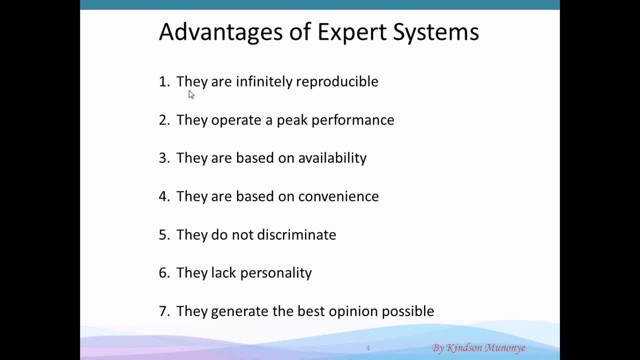 A human expert cannot duplicate himself into different locations, But an expert system can be replicated in different locations to handle as many users, as many problems as possible. This is not possible with humans And that is why it's important. That is why they are infinitely reproducible. 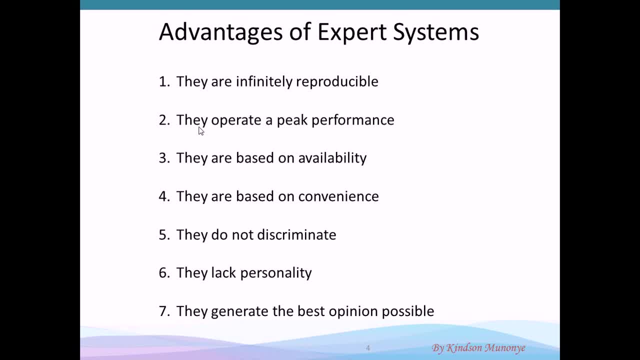 That is one of the core advantages of expert systems. And let's look at number five. They do not discriminate. A human expert may be swayed by the person he sees: a relative, a non-relative, somebody from his race, and so on. 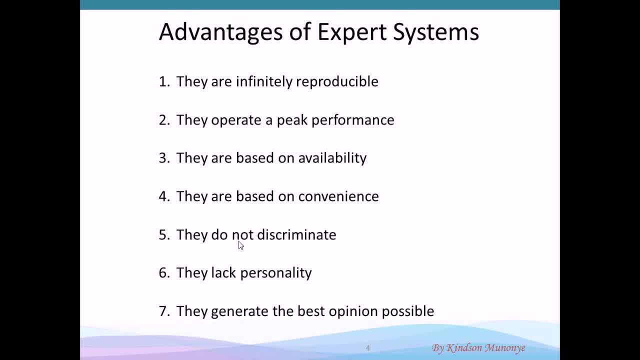 But an expert system does not discriminate. Number three: always available. Okay, So these seven points. try to understand them. These are what makes expert systems unique, And that is why we need expert systems. in our modern world, We have some expert systems. 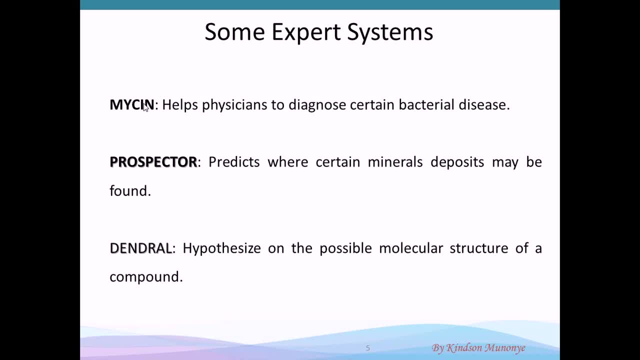 I would like you to just do a Google search of these three expert systems. We have the Mycene that was developed sometime using the medical field And helps doctors to diagnose bacteria, Diagnose bacterial diseases. They will have Prospectal Helps geologists to predict where mineral deposits may be found. 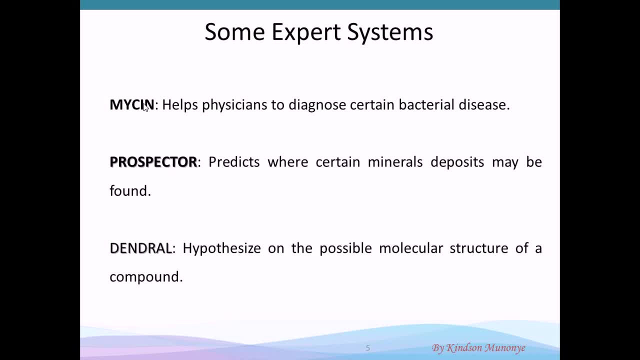 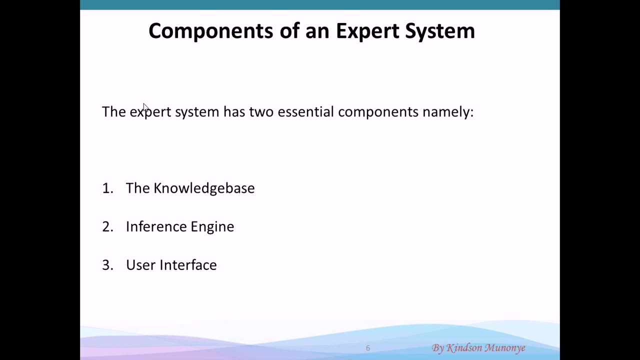 They will have. Dendral Helps to hypothesize on molecular structure of a compound. So this is just. you take some time to go to Google and search and find what all this is all about. Let's proceed to the next slide Now. there are three components of the expert systems. 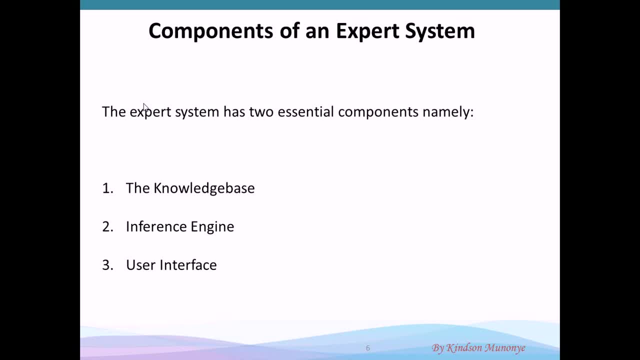 The knowledge base, the inference engine and the user interface. But in this presentation we are going to focus on one: the knowledge base and the inference engine. The third one, the user interface, I'm not going to cover it here. 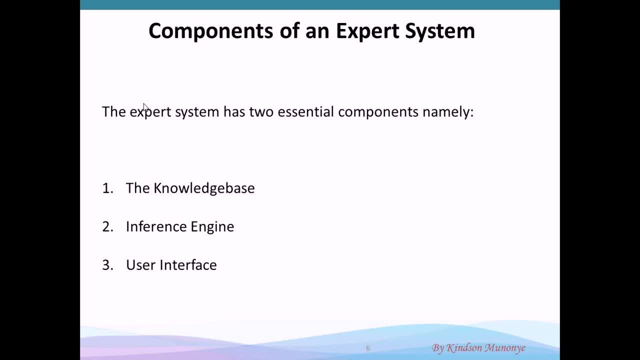 But take note, the user interface is simply an interface between the user, the human user, and the computer In form of a screen, a display, Input, output device and what have you. So our presentation focuses on the knowledge base and inference engine. 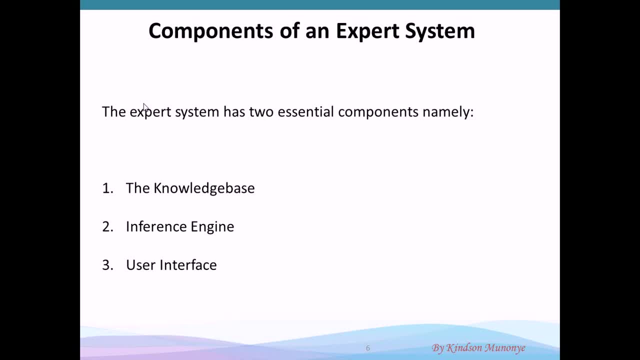 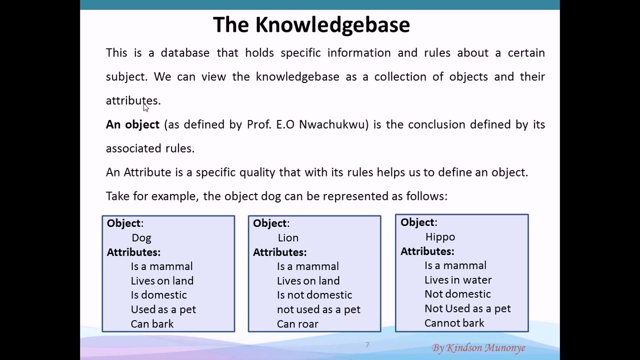 So I'm also going to add some other components, like database, But I think these three are the core components of the expert system. So what is the knowledge base? It is a database, A repository of information and rules about certain subjects. So we can look at the knowledge base as collection of objects and attributes. 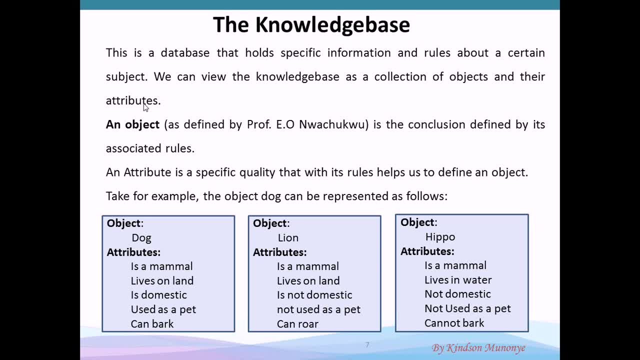 What is an object, Defined by Professor IO Machuko, is the conclusion defined by its associated rules. Then attributes are characteristics of objects, Specific qualities that, with each rule, help us to define an object. So we have some examples here Of what objects might be. 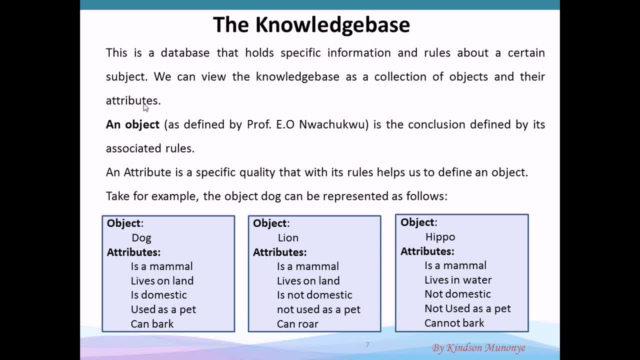 And take note that the knowledge base is a collection of objects and the attributes. Let's take, for instance, dog. Dog has attributes like is a mammal, lives on land, is domestic, is user's pet and it comes back. So these attributes mentioned here is not definitive. 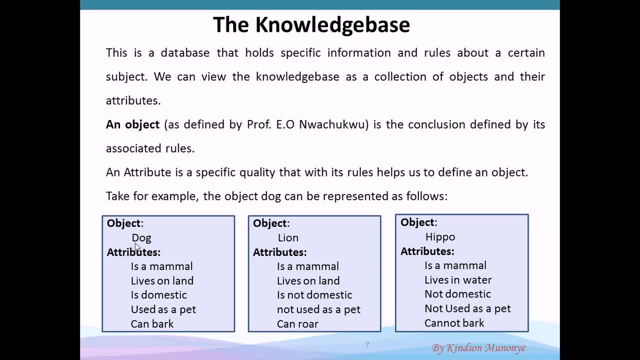 They can be other attributes, But sometimes not In the knowledge base. of course, there must be a finite number of attributes that are assigned to a particular object in the knowledge base. So getting it clear, a knowledge base is a database, a collection of information of objects and the attributes. 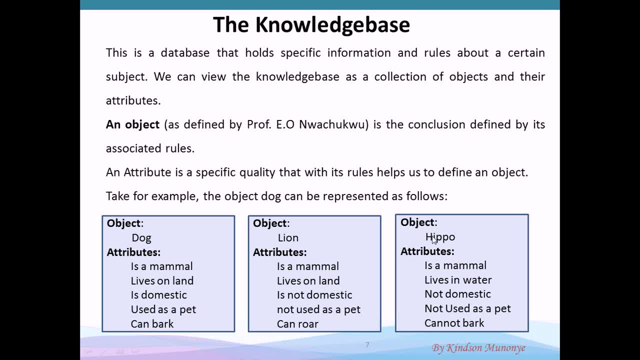 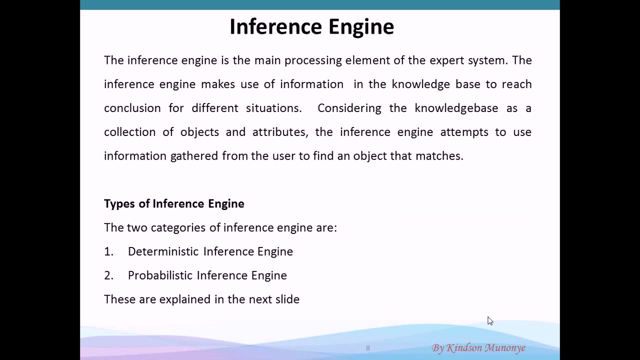 So we have, for instance, we have hippo. We have is a mammal, It lives in water, It's not domestic, It's not user's pet, It cannot bark. OK, That's the attributes for a hippo. 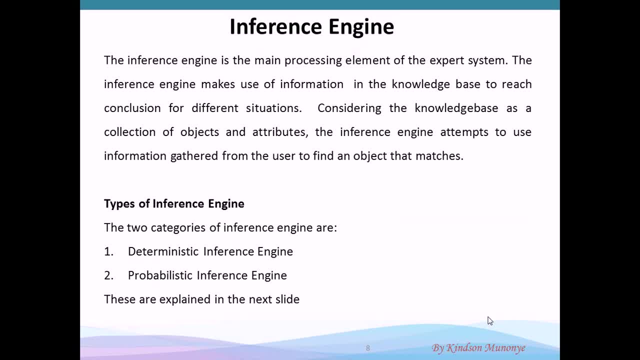 Now, the next component of the inference engine is the of the expert system, is the inference engine? Now, what is the inference engine? The inference engine can be described as the processor of the expert system. It makes use of the information from the knowledge base to reach conclusion. 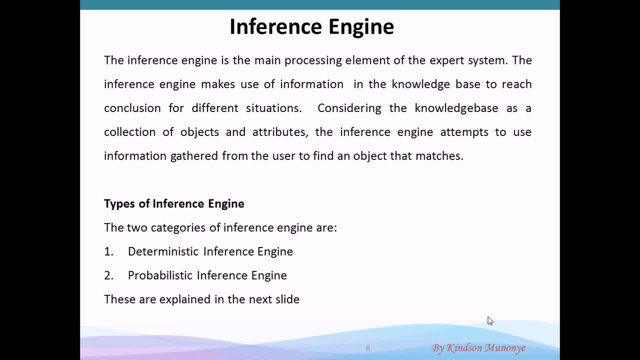 OK, Now take note that there is information in the knowledge base. There is also information that is gathered from the user. OK, So, getting this information from the user, the inference engine decides, attempts to find objects in the knowledge base That matches the information gathered from the user. 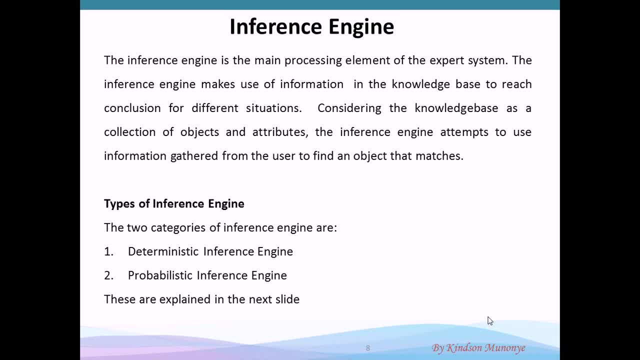 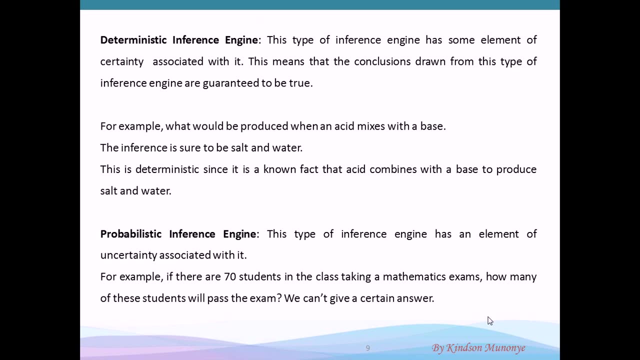 OK, I think that's clear enough. So we have two types of inference engine: One, the deterministic inference engine and the probabilistic inference engine. I explain this in the next slide. If an inference engine is deterministic, then there is element of certainty associated with it. 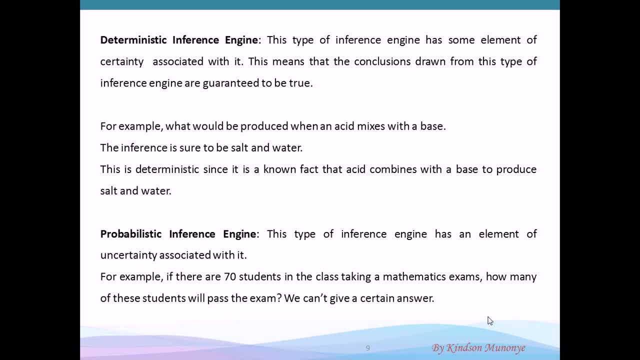 What do we mean? It means that the decision reached by this inference engine is sure, is certain, is guaranteed to be factual. OK, For instance, what is the result of an acid combined with a base? An acid combined with a base produces salt and water. 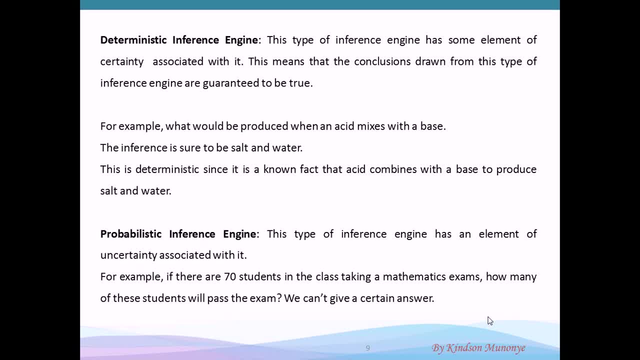 There are no two ways about it. It's the fact, It's a verified way, It's a well-known fact, that does not change. OK. So if inference engine reaches this kind of decision from known facts that is certain, has element of certainty, then we say it is a deterministic inference engine. 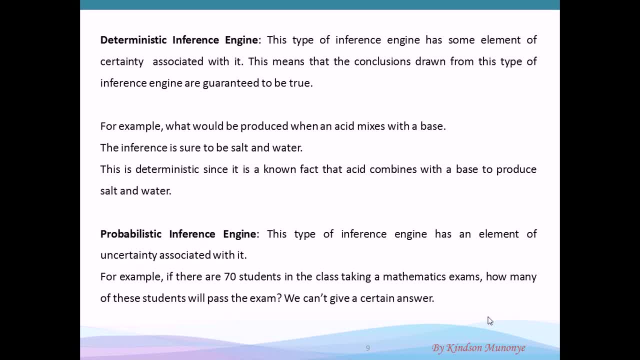 Then the next one is a probabilistic inference engine. An inference engine is probabilistic when there is element of uncertainty associated with decisions reached by this inference engine. For instance, if there is a class of 70 students and the question is: they are writing an exam or they are taking a test, how many of these students will pass the exam? 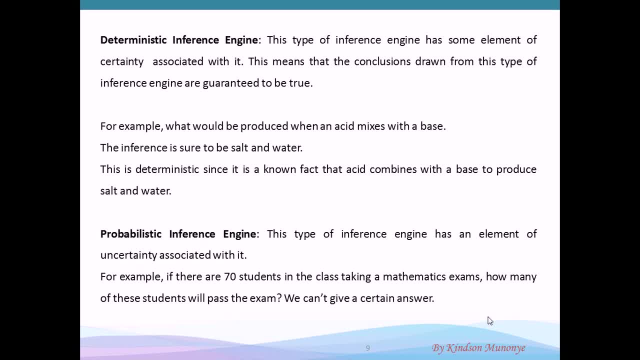 The answer is not clear, but some conclusion may be reached. OK, So some inference can be made based on the previous performance of the class. Some inference can be made or based on the difficulty of this exam of text. an inference can be made, say, and maybe half of the students will pass, maybe 70%. 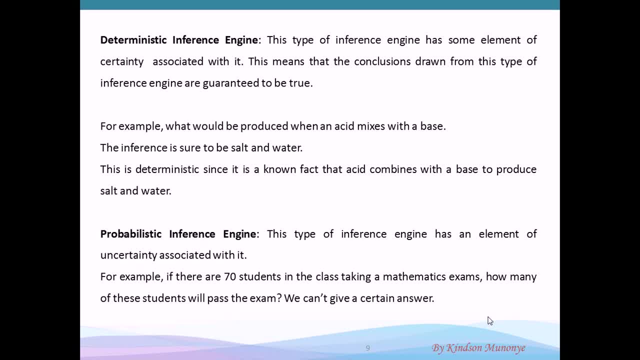 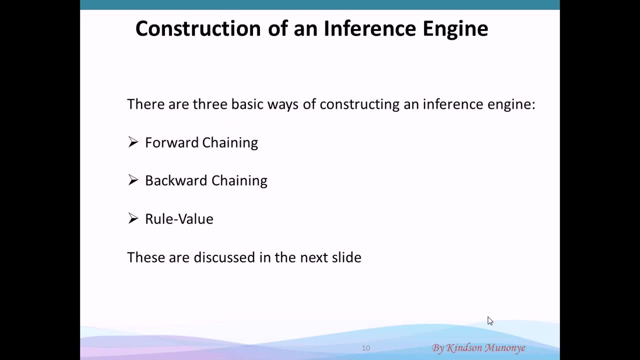 But these decisions are not deterministic. They are probabilistic, meaning that they are based on probability And has element of certainty And has element of uncertainty associated with them. Let's proceed. We have the next topic. we are going to discuss construction of an inference engine. 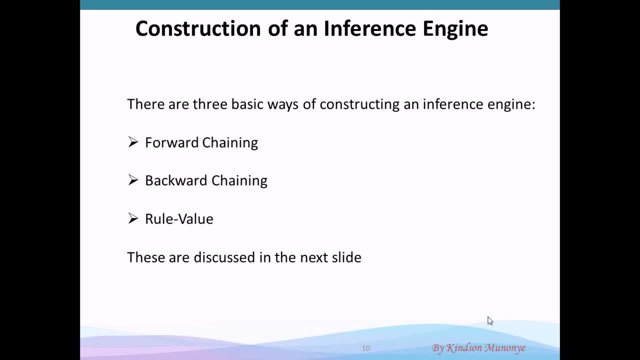 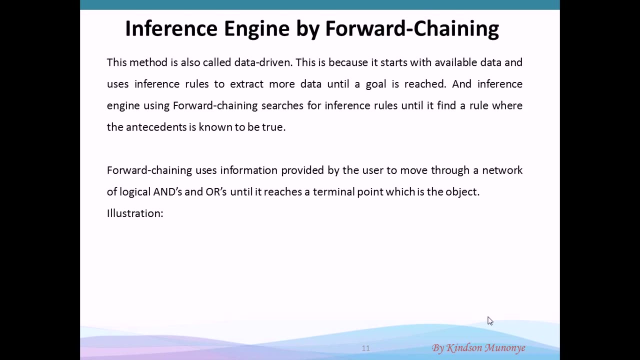 Now there are three basic ways to construct an inference engine. The first one is the forward chaining, The second is the backward chaining, And then we have the rule value or rule-based inference engine. What is the difference? I think let's look at the difference. 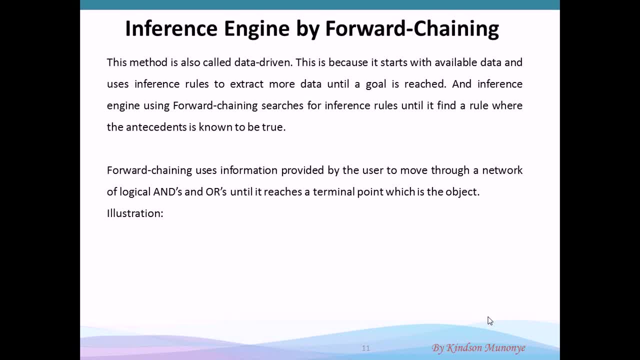 We take the first one inference engine constructed by forward chaining. Remember we say that the knowledge base is a collection of objects and associated attributes and rules. OK, Now the forward chaining inference engine starts with the attributes or the data and uses inference rules to get more data and reach a conclusion. 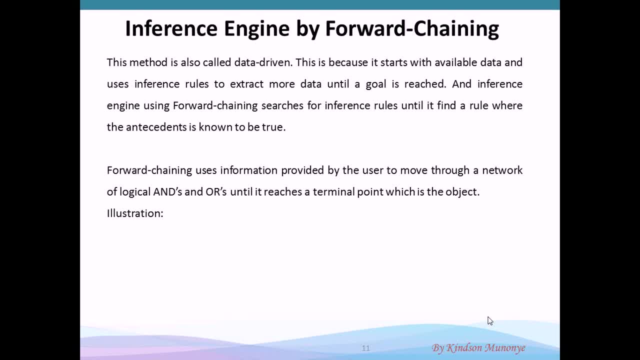 OK. So the forward chaining inference engine starts with the data. OK, It gets more data and then, based on this data, it draws a conclusion. For instance, let's take for instance we have: is it a domestic animal? Yes, Does it live on land? 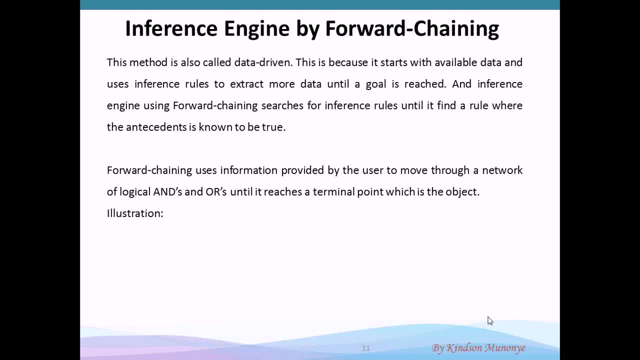 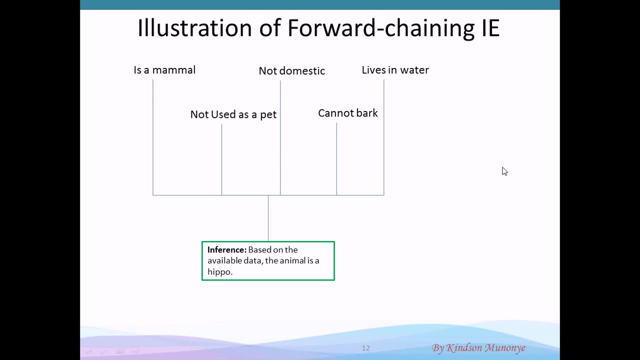 Yes. Is it a mammal? Yes, Does it bark? Yes, Then it is a dog. OK, So the goal or the object. you reach this conclusion at the later end, after using the rules, And that is what we have here. 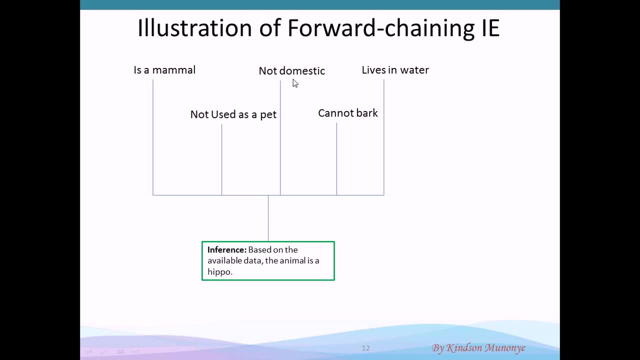 We have the data is a mammal, not domestic, OK, Not used as a pet, cannot bark and lives in water. Based on this data, we draw a conclusion or make an inference: the animal is a hippo, Because the data we have matches the characteristics or the attributes of a hippo. 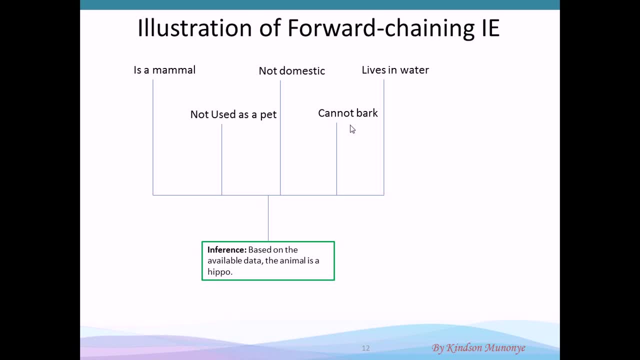 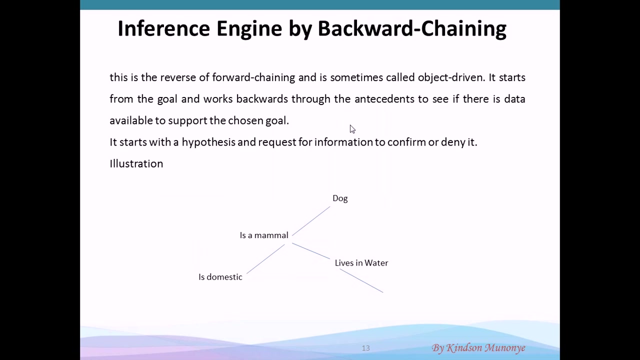 So the forward chaining inference engine takes data and then makes inference to find an object. It gets data and finds the object that matches the data. Now the backward chaining inference engine is the opposite. What the backward chaining inference engine does is it starts with the object. 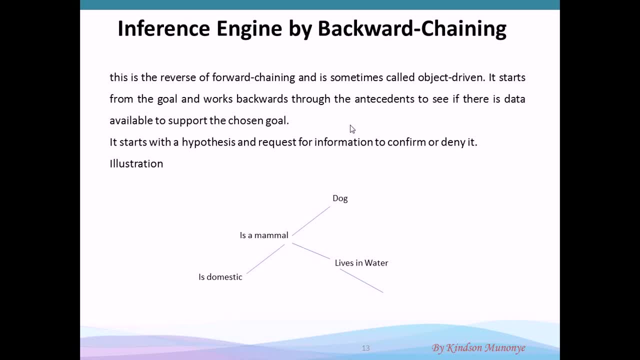 It takes a blind guess. OK, Oh, Is it a dog? Is it a dog? Is it a mammal? Yes. Does it live on land? Yes. Is it domestic? Yes. Is it used as a pet? Yes. 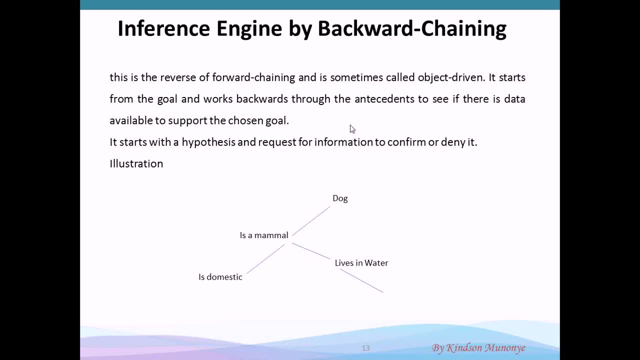 Oh yes, Sure, My guess is right: It is a dog. So that is how it works. OK, Let's go to the next question. Is it a dog? Yes, Yes, That is how the backward chaining works. It makes a guess and starts getting the data to either confirm or deny. 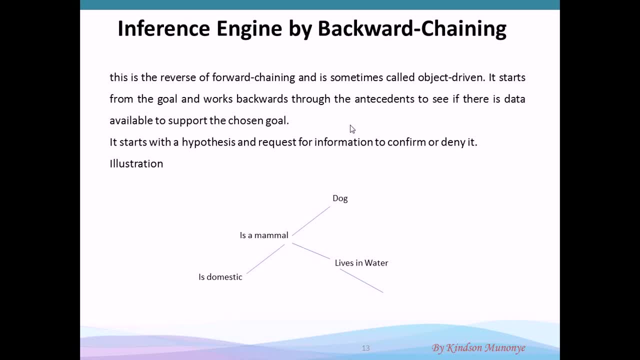 So if we have this inference engine guessing at the initial time is a dog And then the data it gets is it lives in water, What would be the inference? The inference would be: it is not a dog. and then it starts all over or goes another direction. 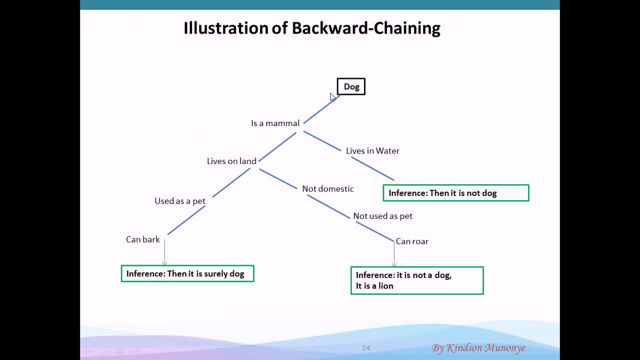 So this is what I illustrate here. We have The guess or the hypothesis says it is a dog. Then it gets data to either confirm or deny. Is it a mammal? Yes, Lives on land. Is it used as a pet? 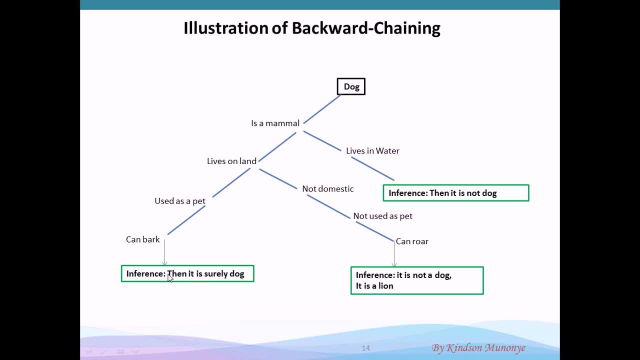 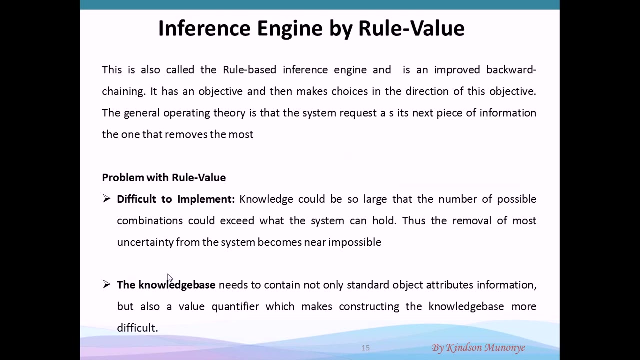 Come back. The inference says it is surely a dog. So this is backward chaining. Now we have discussed forward chaining. We have discussed backward chaining And now the next one we are going to discuss is the rule of value. We are not going to spend much time here. 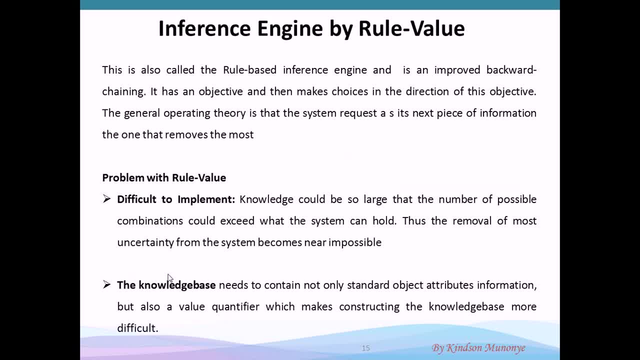 But the rule of value is improved backward chaining. What it means is it makes a hypothesis And then asks questions. that leads it to its objective. OK, So The data it gathers. It gathers data that tends to confirm that the hypothesis is correct. 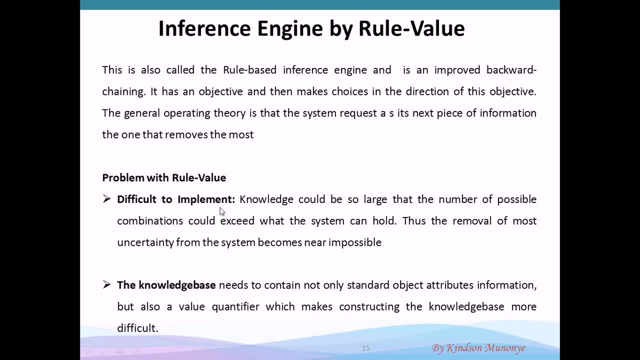 OK, So We have about two problems with it Difficult to implement. The knowledge base for this type used to be very, very large. Then here the knowledge base needs to contain not only standard object attributes information, But also value quantifiers, which make constructing the knowledge base more difficult. 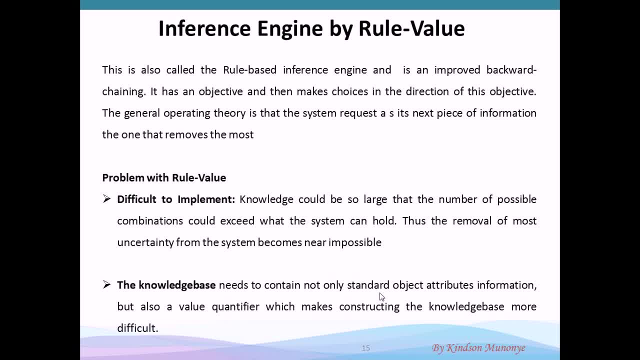 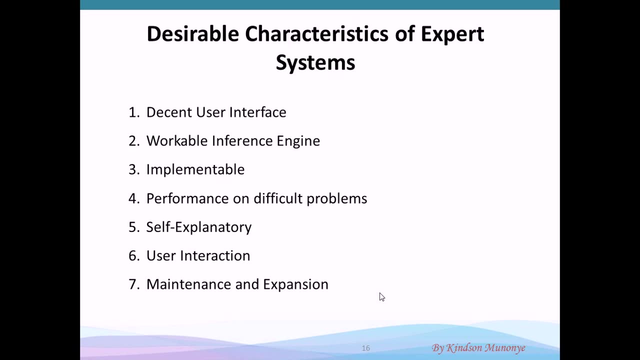 So Here is the rule of value. Just take note that there are There are three inference engine methods: Forward chaining, Backward chaining And the rule of value. So we have characteristics of X-pass systems. There are seven of them. 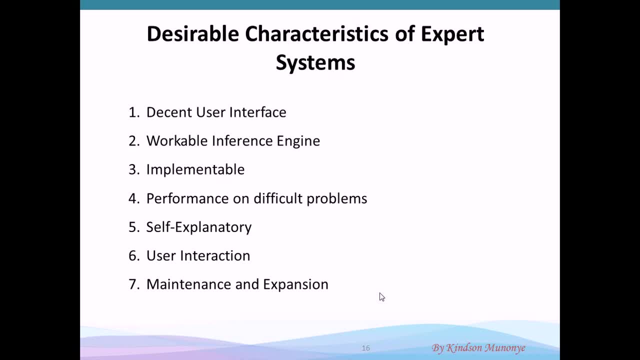 I am not going to explain everything, But maybe you pause this video, Take a pen and a paper, Write all these advantages or characteristics of the X-pass system And then you try to go through So we have the decent user interface. It should be able to have a friendly interface. 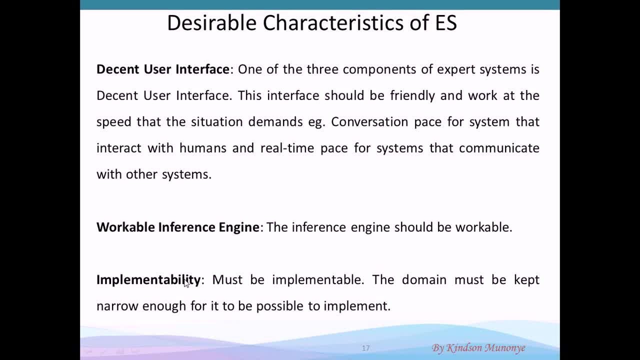 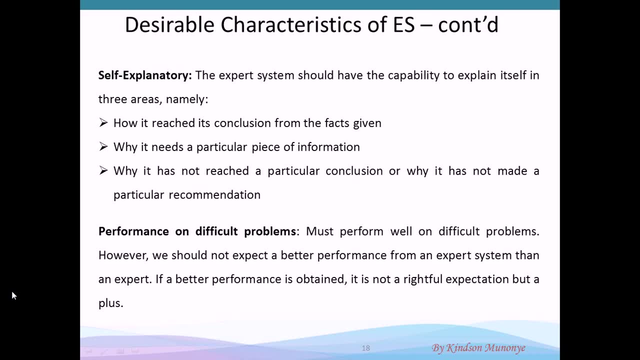 To communicate or interact with the user, Then it should have a workable inference engine. It should be implementable, Not too complicated. It should be self-explanatory. An inference engine should give a feedback on how it reached a conclusion. It should be able to backtrack to tell the user how it reached a conclusion. 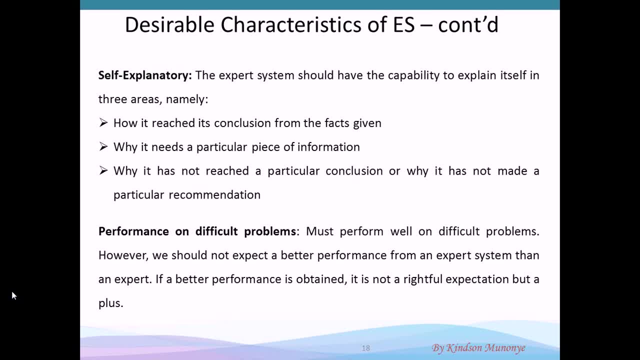 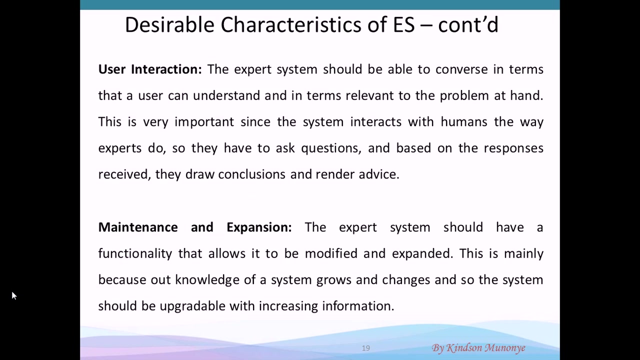 Then why it needs a particular piece of data And why it has not reached a particular conclusion, As the case may be, Then an X-pass system should handle difficult problems. It should perform well on difficult problems. User interaction should not be too complicated for a user to use. 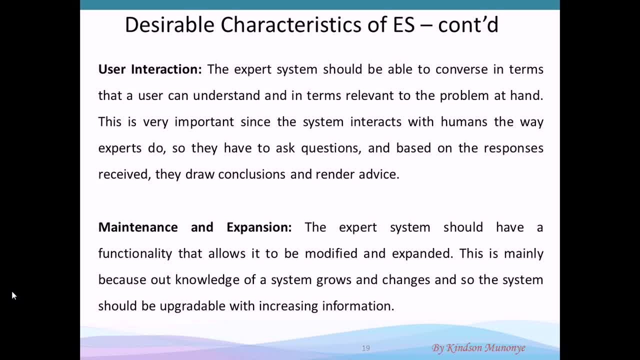 When it comes to interaction, It should do so in a pace That humans can follow. Maintenance and expansion: An X-pass system should be upgraded, Should be expandable, Can be modified, Can be scaled up, And so on. Alright, 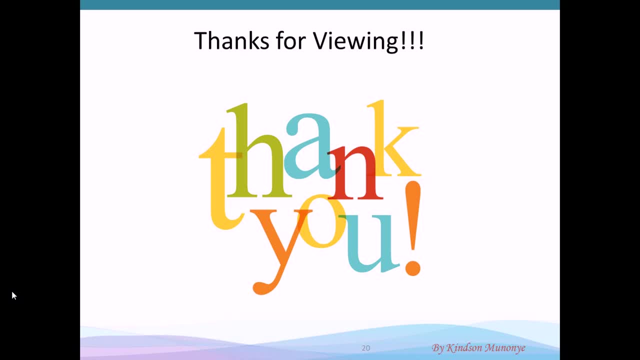 I hope you enjoyed my video on X-pass systems. If you find this video informative, Please give me a thumbs up, Subscribe to my channel And once again, I would like to thank you for viewing.